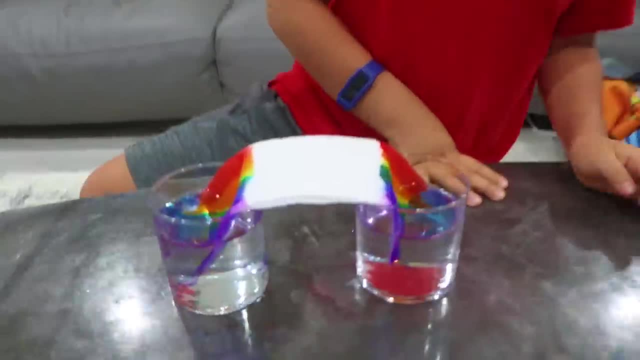 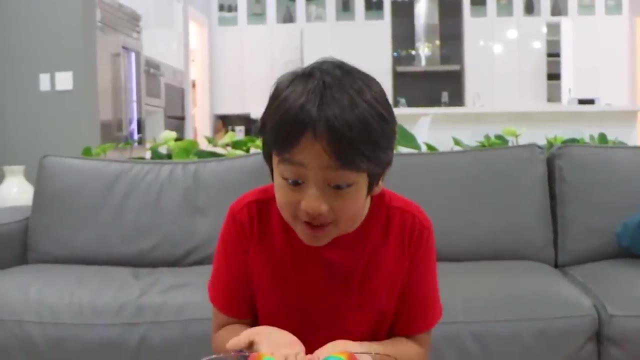 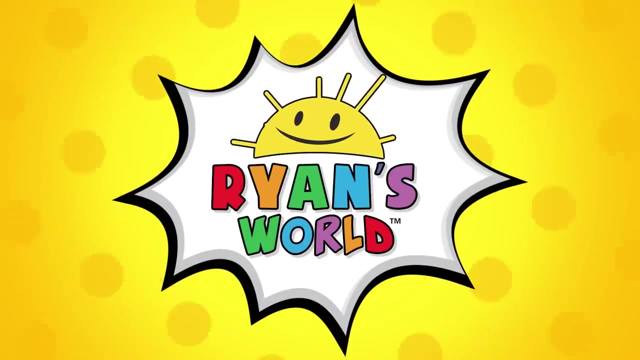 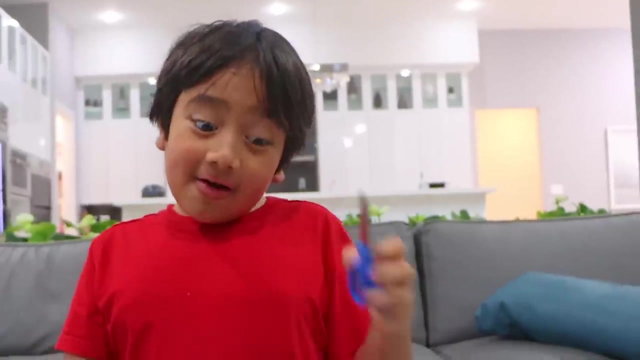 Now we wait. Let's watch the rainbow form. Look, it's already forming a little bit. Well, guys, did you see? We made our own rainbow. Welcome to Ryan's World. Hey guys, today we're gonna grow our own rainbow. All you need is a paper, towel, scissors, markers. 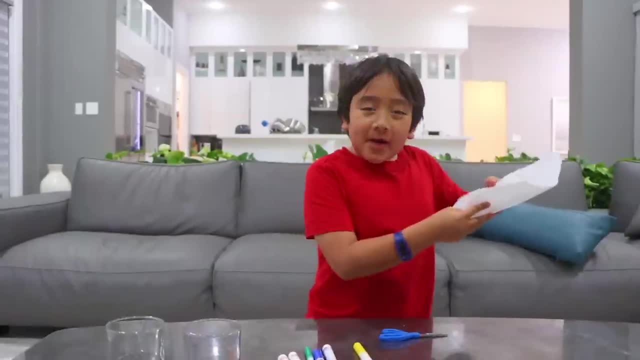 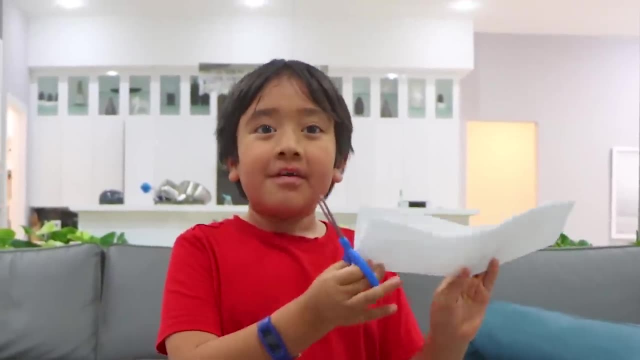 and cups with water. First, using your paper towel, you're going to fold it in half, and then we're going to cut a one-fourth. Don't forget to ask a grown-up for help, and I have mommy here, Hi, Hi. 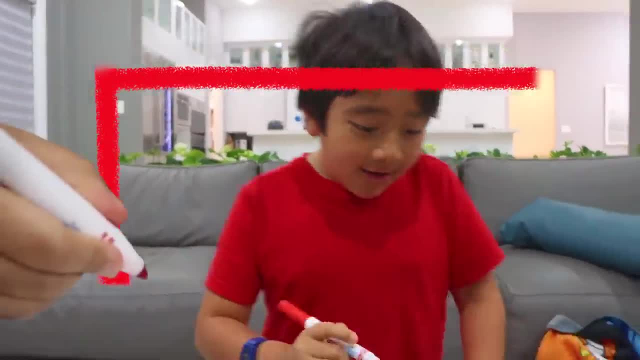 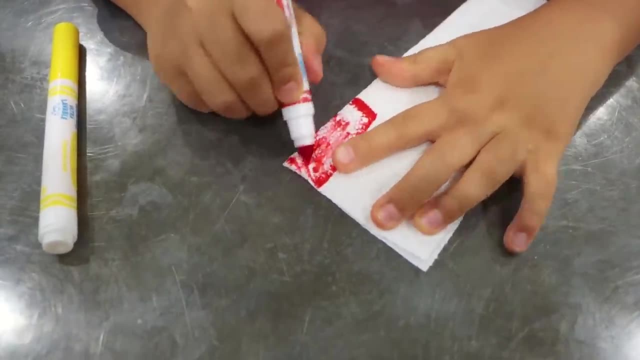 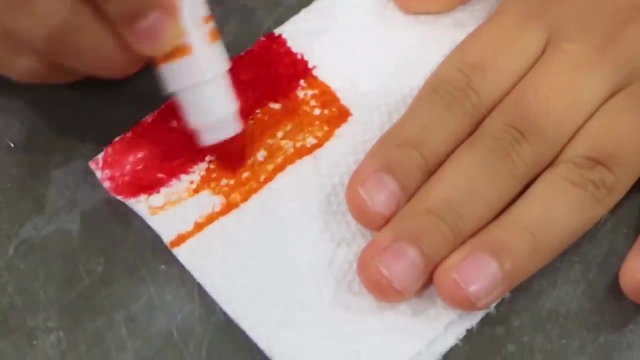 Thanks. So first, with any marker you want, make a rectangle like this: Now let's color it in. The next color in the rainbow is Orange. Put it like this: Now let's fill it in. Next is yellow. Okay, let's fill this in. 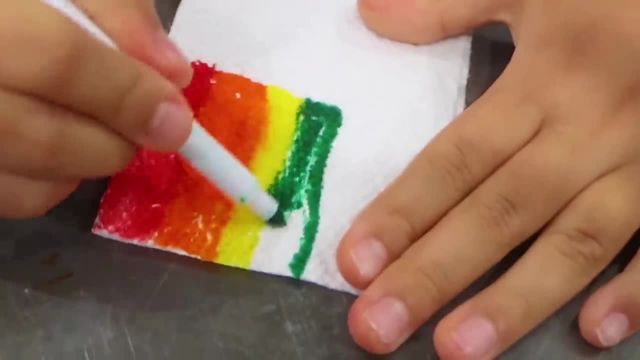 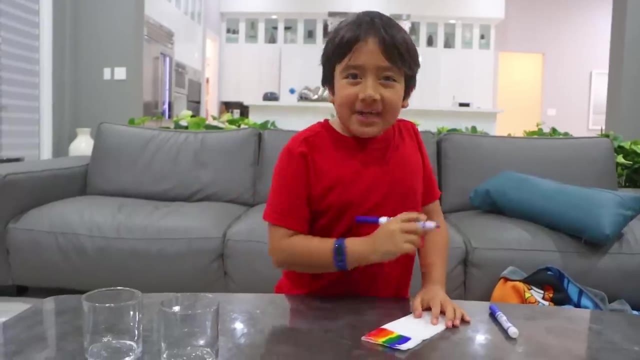 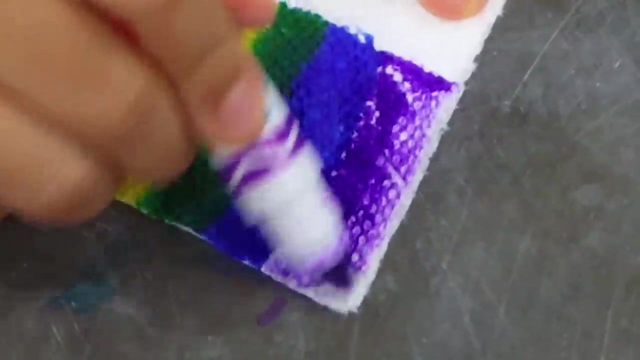 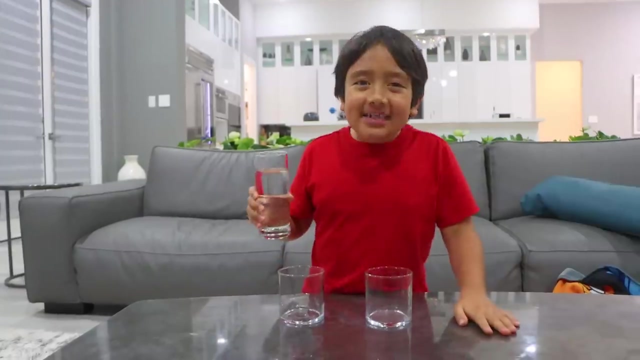 Next is green. Fill it in Green. Next up is blue. We're gonna finish it up with my favorite color, purple. Now do the same thing to the other side. Like this, See, Like. so Next, fill up your two thingies of water. 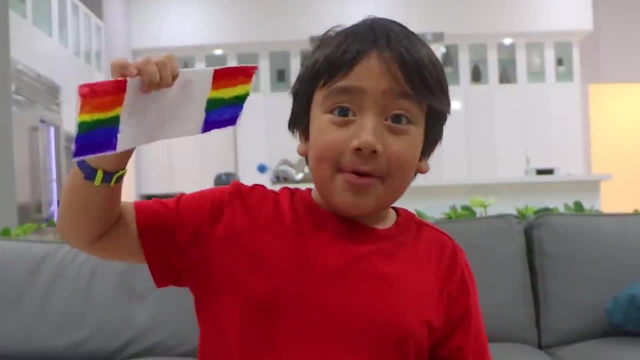 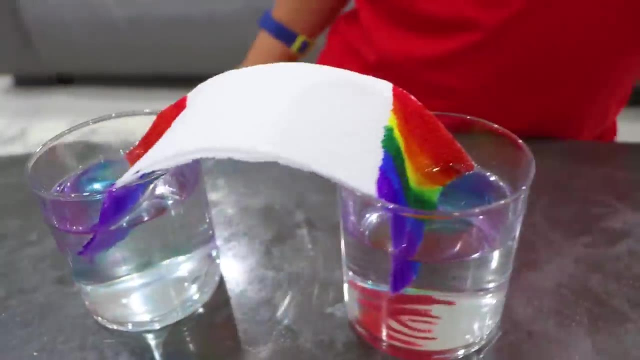 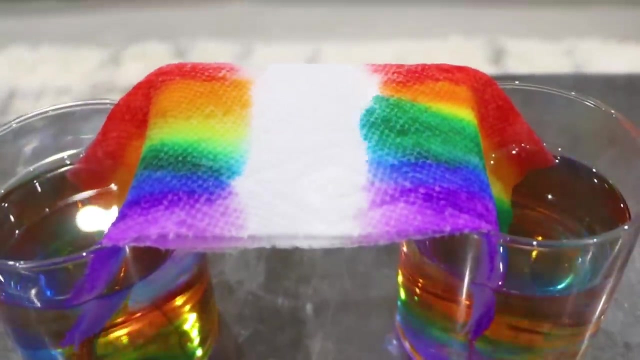 And the second one. Now take your rainbow paper that you drew and put half of both of the sides in the water. Now we wait. Watch the rainbow form. Look, it's already forming a little bit. Whoa, guys, did you see? We made our own rainbow. Whoa, Let's put it right here. 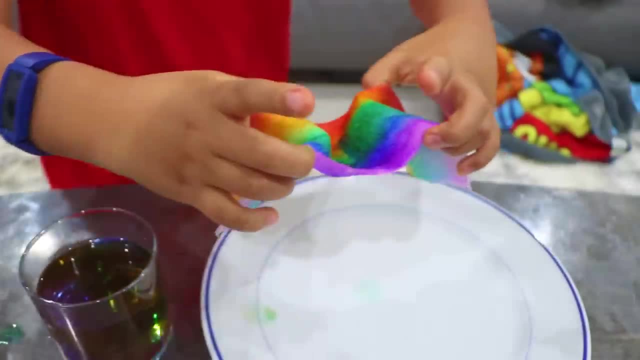 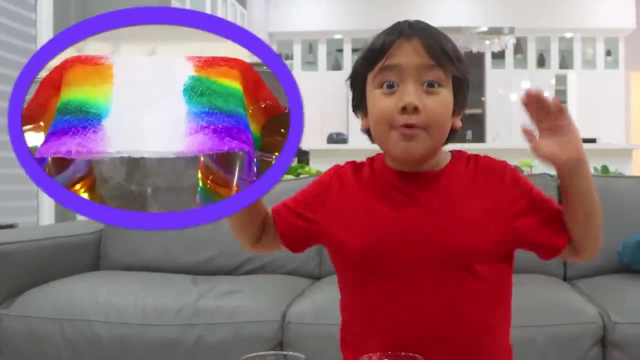 This is so cool. Did you see the marker die? move up the paper towel and touch each other, Because that's called capillary action. Did you know regular plants also use capillary action Because they bring the water from the roots and make it look like a rainbow? 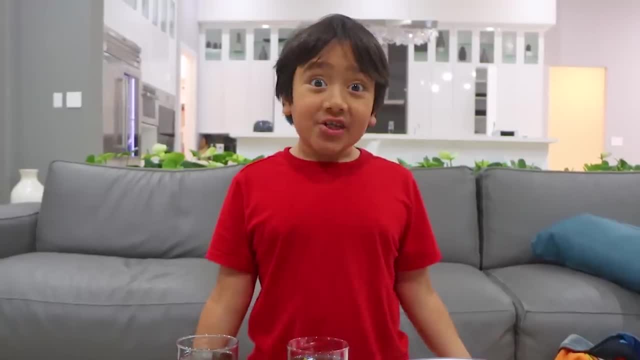 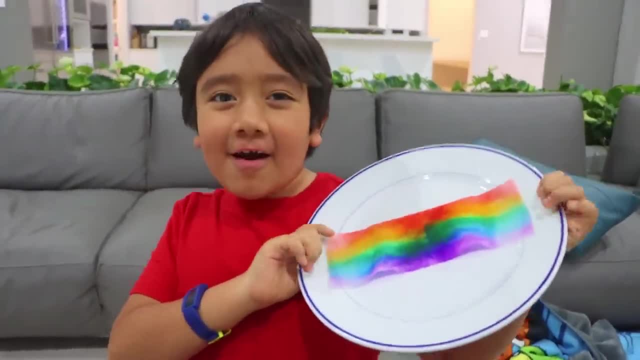 I hope you guys had fun making our own rainbow together. Bye, Remember. always stay happy and rise up. Bye.